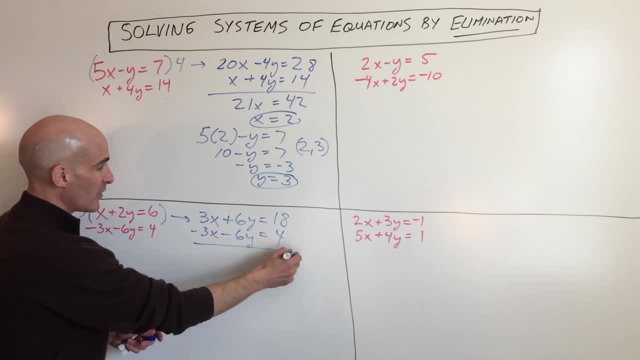 minus 6y equals 4.. And when we add the x's cancel, the y's cancel, We end up getting 0 equals 22.. Now what does that mean? 0 equals 22? That's a nonsense, right? That's a nonsensical answer. 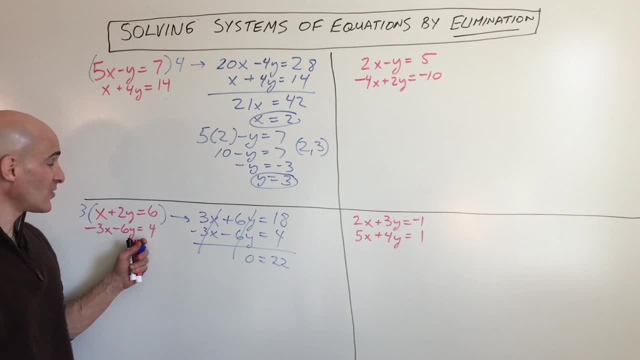 It doesn't make any sense, And what that actually tells us is that these two lines are parallel. So if you were to graph them, they would be like this: They don't cross, So this one. there's no solution, So empty set. 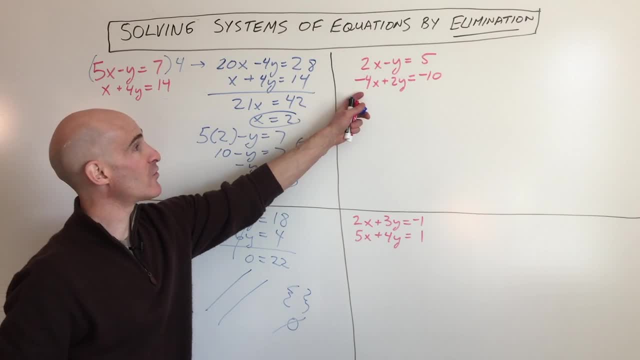 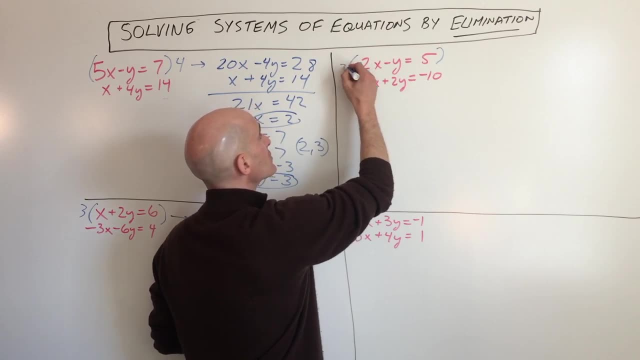 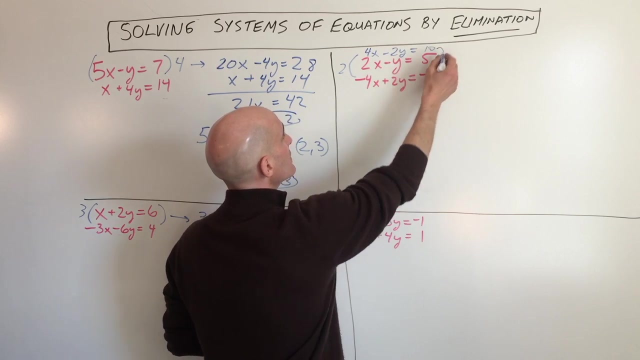 no solution or you can just write no solution. Okay, this next one over here. let's eliminate the y's. We're going to multiply the top equation times 2. So if we do that, we're going to get 4x minus 2y equals 10.. So if we combine the 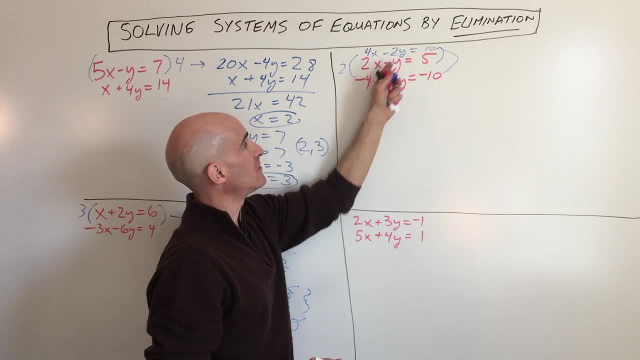 top equation. with the bottom equation you can see the x's cancel, the y's cancel and even these numbers on the right side of the equation cancel. So we're getting 0 equals 0. What that tells us is that these lines are the exact same line. So if you were to graph them, one line would be like: 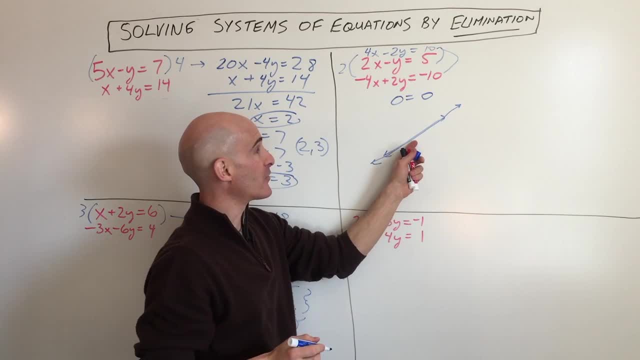 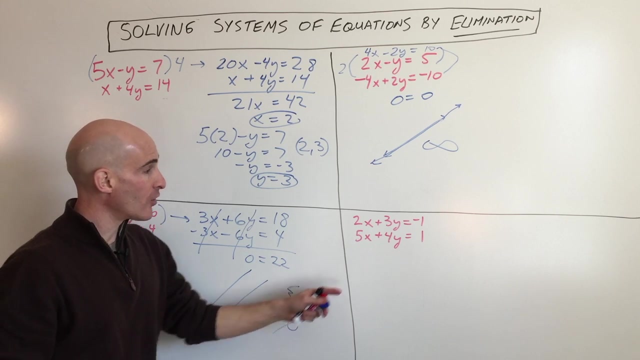 this, The other line would be right on top of that line and they're crossing at an infinite number of points. So this one is, you know, infinite number of solutions, or you could say consistent, dependent, So consistent, dependent. This one over here was inconsistent, Okay, and then these other. 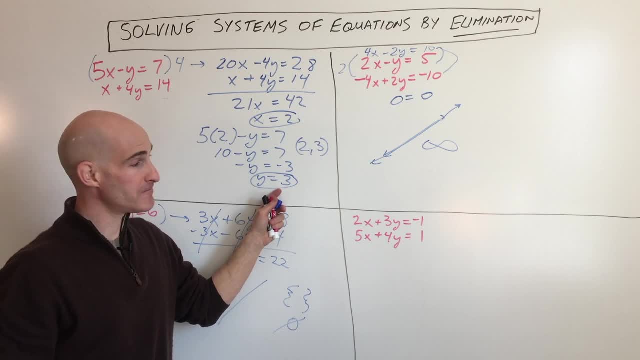 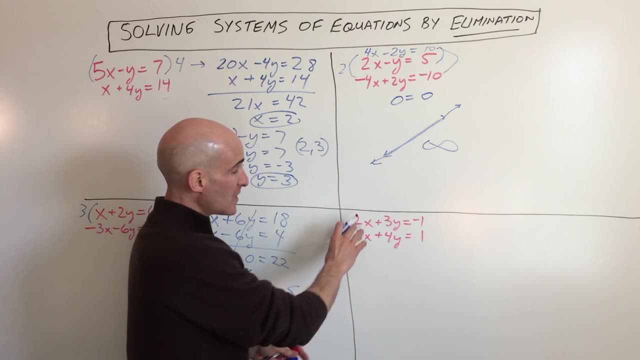 ones that we're working on. this is consistent, independent. Okay, so this one here is a little different example. Okay, so this one here is a little different. Okay so this one here is a little different. And here we're going to have to multiply both equations so that we can eliminate one of the 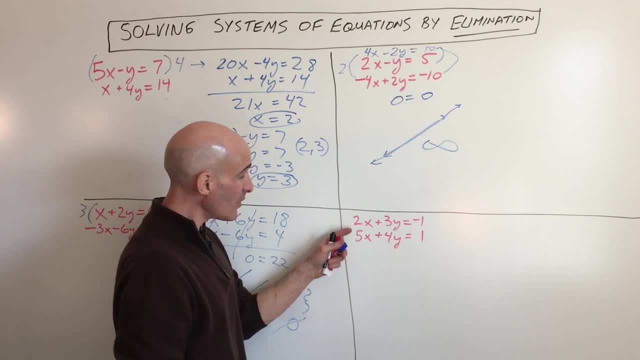 variables. So let's just say we want to eliminate the x's. What does 2 and what does 5, what do they both go into? evenly 10.. That's the lowest common multiple. But let's make one of them negative: 10. 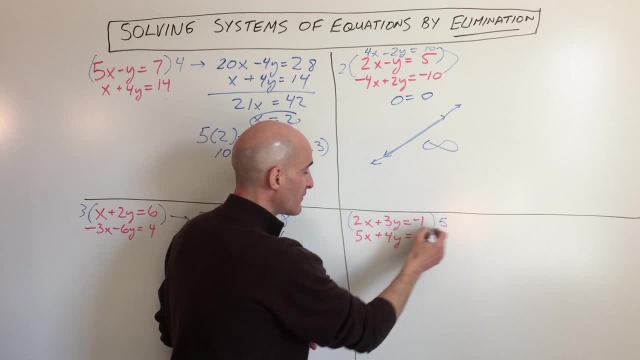 and one positive 10.. So we're going to multiply this top equation times 5, the bottom equation times negative, 2.. Okay so if we do that we get 10x plus 15y equals negative 5.. In the bottom equation we get negative. 10x minus 8y equals negative 2..